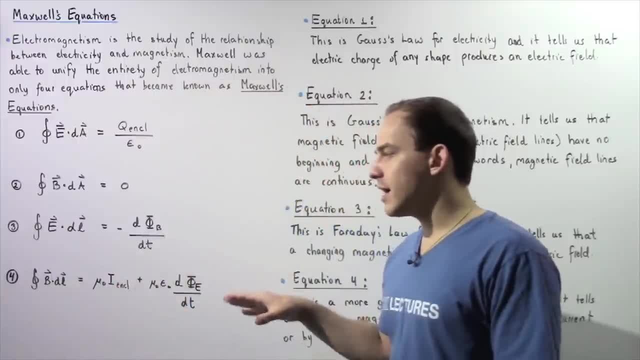 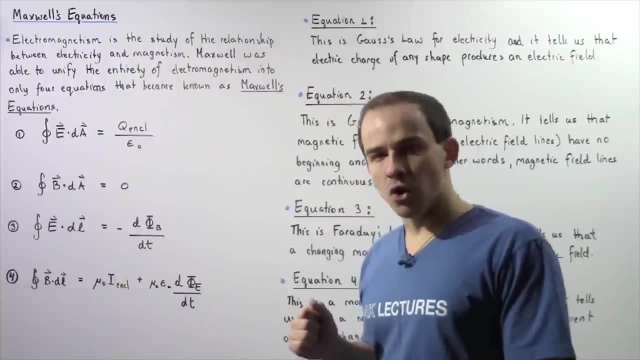 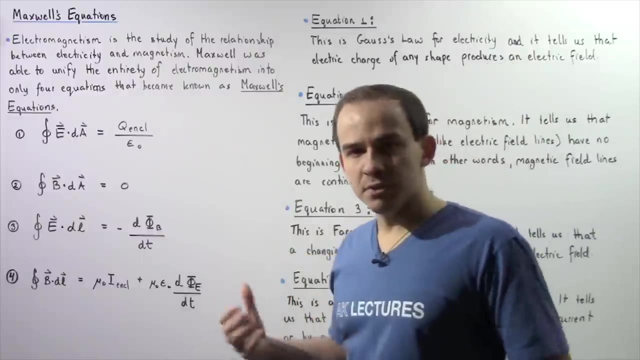 Now, equation 4,, which we're going to discuss and derive in the next lecture, is known as the general form of Ampere's law. So let's go through each one of these equations and let's summarize the implication of each one of these equations. 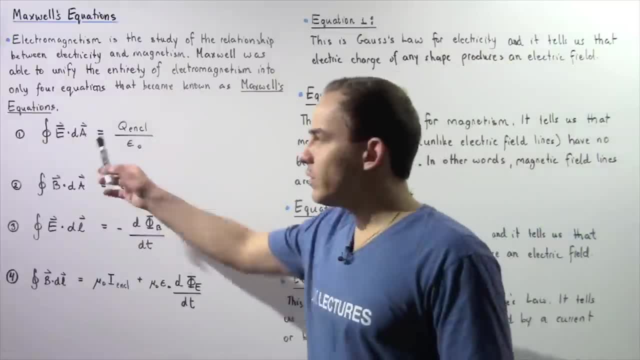 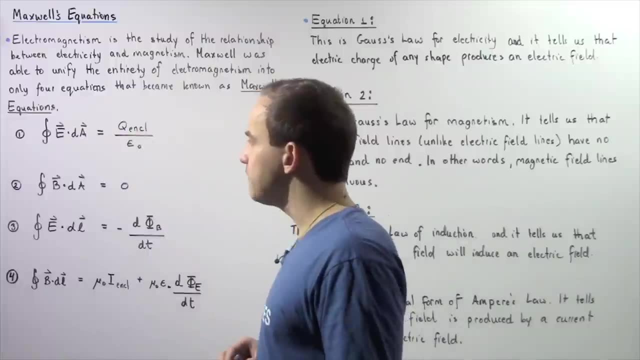 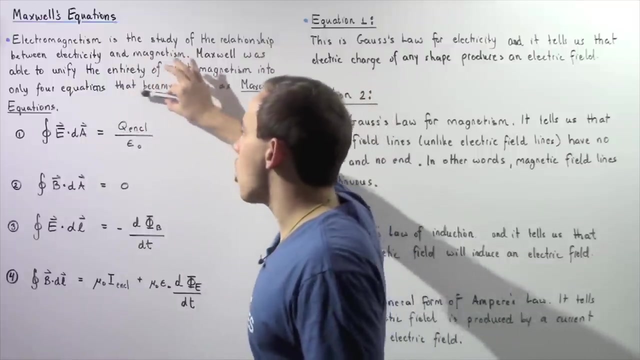 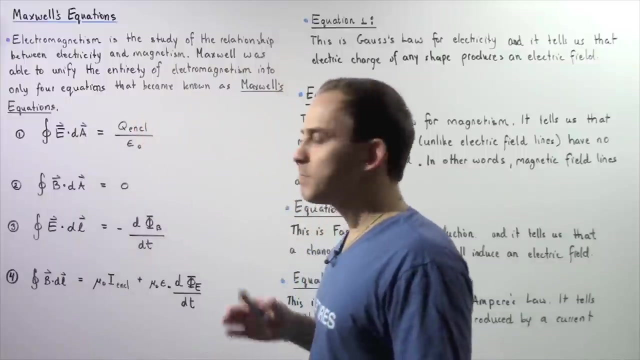 So let's begin with equation 1.. So equation 1 tells us that the closed integral of the dot product of the electric field vector and our infinitely small area vector dA is equal to the total charge enclosed in our chosen surface, divided by the constant known as permeativity of free space. 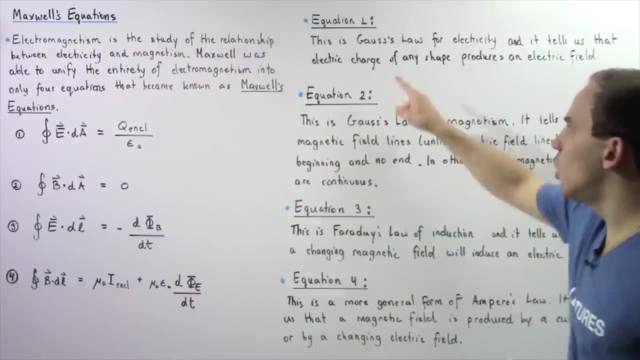 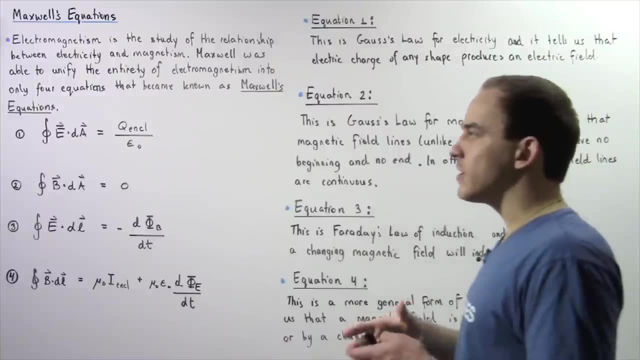 So this equation, once again, is known as Gaussi's law for electricity, and it tells us that any time we have an electric charge, So this equation, once again, is known as Gaussi's law for electricity and it tells us that any time we have an electric charge, 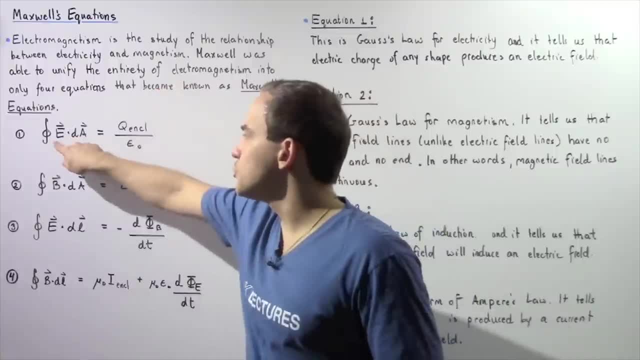 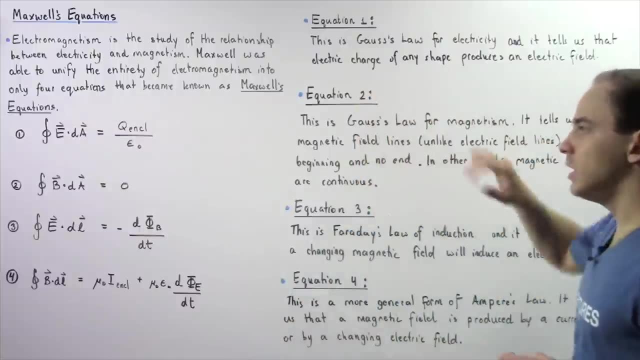 that electric charge will produce an electric field. So it connects the concept of charge and electric field. Now let's move on to equation 2.. So equation 2 is known as Gaussi's law for magnetism. It tells us that magnetic field lines, unlike electric field lines, have no beginning and no end. 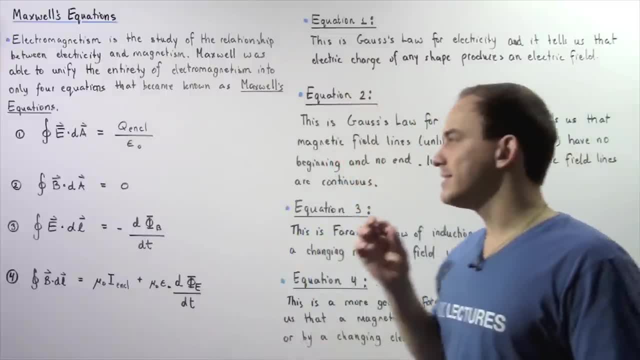 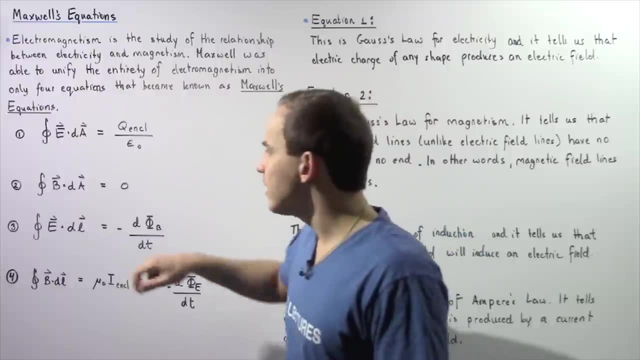 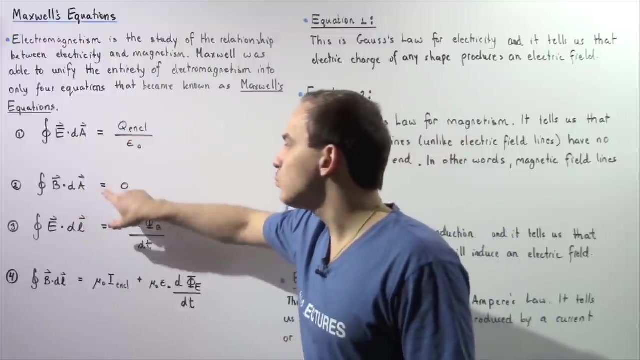 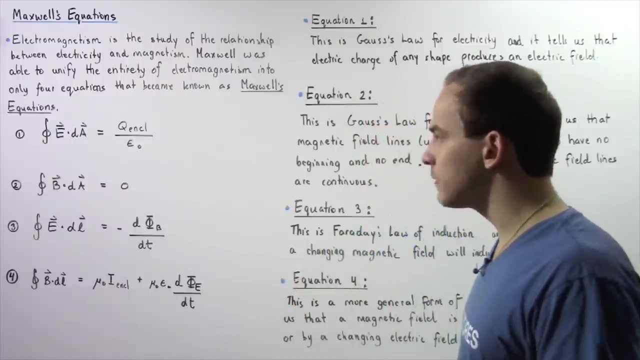 It tells us that magnetic field lines, unlike electric field lines, have no beginning and no end. Magnetic field lines form continuous loops and that means that if we take the closed integral of the dot product of our magnetic field B and our infinitely small vector dA, that will equal zero, because the net magnetic flux through our chosen Gaussian surface will be zero. 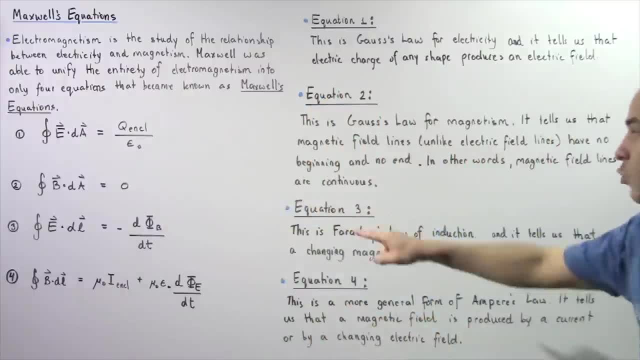 Now let's move on to equation 3.. Equation 3. Equation 3 is known as Faraday's law of electromagnetic induction, and it tells us that a changing magnetic flux as a result of a changing magnetic field will induce an electric field as described by the following equation: